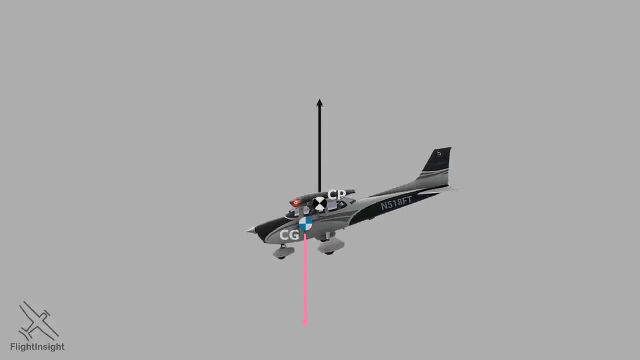 counteract each other. In fact, the stronger the lift and weight, the greater this pitch-down tendency becomes. An aircraft can maintain level pitch attitude thanks to its horizontal stabilizer, which resists the pitch-down movement by exerting a downward force on the tail, which we call. 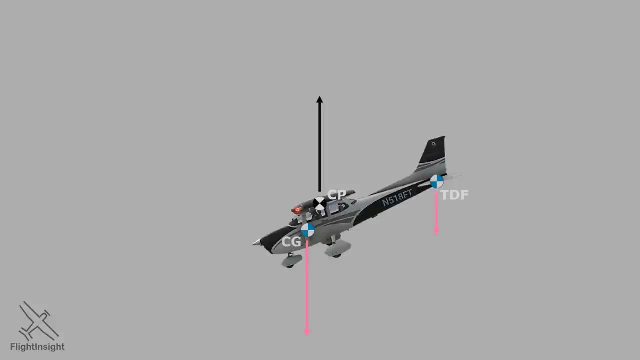 tail-down force, or TDF. So a well-loaded and designed aircraft will have these three forces distributed something like this. Notice, though, that in addition to weight moving downwards through the CG, we also have a second tail-down force, creating a downwards force. This adds to the effective weight of the aircraft. 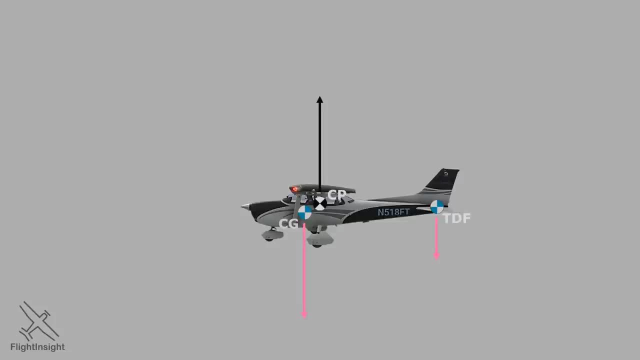 which will have to be counteracted with lift. So in order to maintain equilibrium, our lift will have to match not only the weight moving through the CG but the tail-down force as well, So it'll have to become larger. We can increase lift by increasing angle of attack, So as we fly through 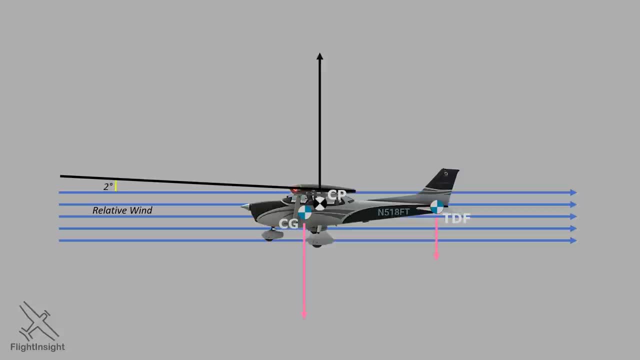 the relative wind we may have an angle of attack of, let's say, 20 degrees, So we can increase lift by increasing angle of attack. We know that if we increase weight we'll need to increase lift by increasing angle of attack. But if we don't increase weight and instead move that center of 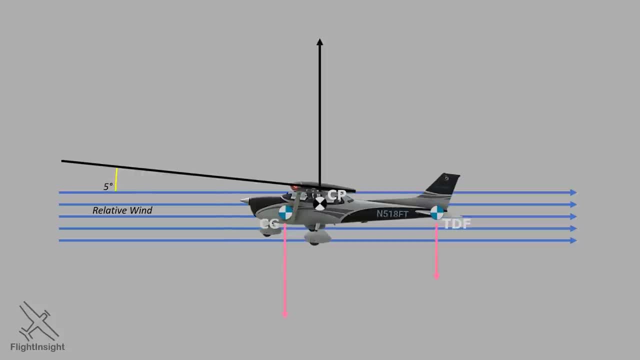 gravity forward a bit, let's say by having a backseat passenger come squeeze up front with us. that pitch-down tendency will become greater and we'll need greater tail-down force to balance it. This will require more lift and hence a higher angle of attack. 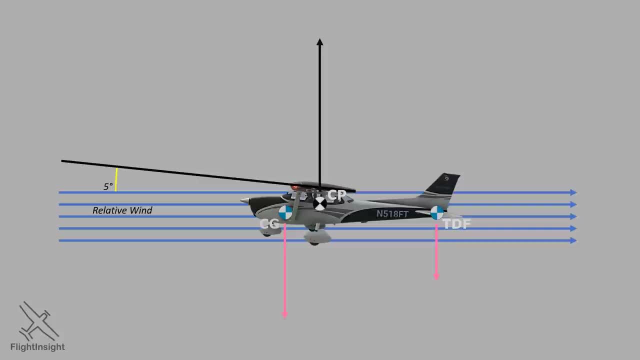 Why is this a good thing to have the CG and CP in different locations? Well, consider what happens in a stall. We pitch up to our critical angle of attack. A stall is a rapid drop and lift. If the center of pressure is the point, we attach the string to the. 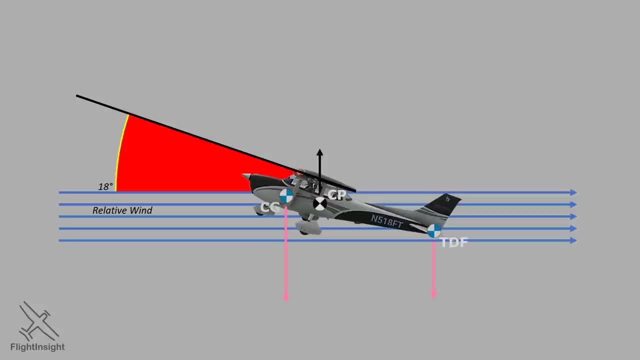 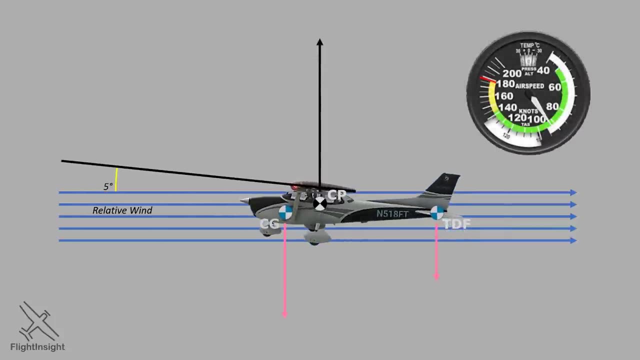 top of the aircraft. we might think of the stall, like we're cutting that string Without much of that lift. the aircraft rotates around its forward center of gravity, pitching down, decreasing angle of attack and helping to break that stall. This is a stably loaded aircraft, So we fly with the center of gravity. 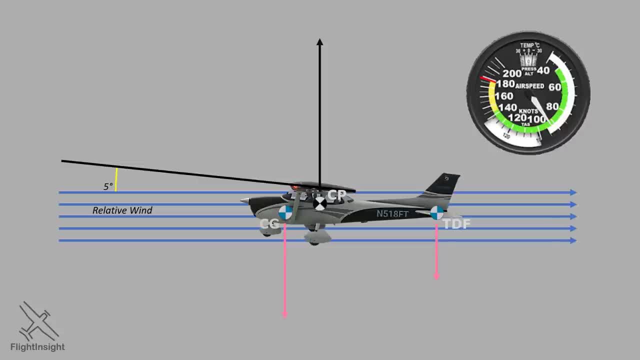 in front of the center of pressure to increase our stability. What's the catch? As we said, with this forward CG, our angle of attack has to be a bit higher to counteract the extra tail-down force. Increasing angle of attack adds drag, specifically induced drag. Remember you can't get something for. 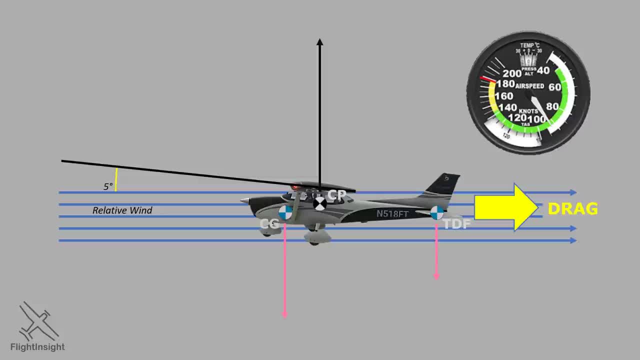 nothing in physics, So we might be flying around 90 knots with this distribution of forces and angle of attack. We could theoretically fly at a zero angle of attack if we moved some weight rearwards and brought the CG right on top of the center of pressure. This would require almost no tail-down. 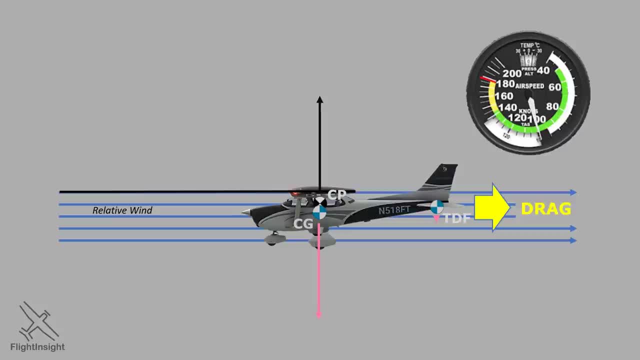 force and our drag would be reduced. For the same power setting, we could fly faster. So a more rearward center of gravity could be more fuel efficient and or allow us to fly faster In a small enough aircraft. I can actually pick up a few extra knots of airspeed just by sliding my seat. 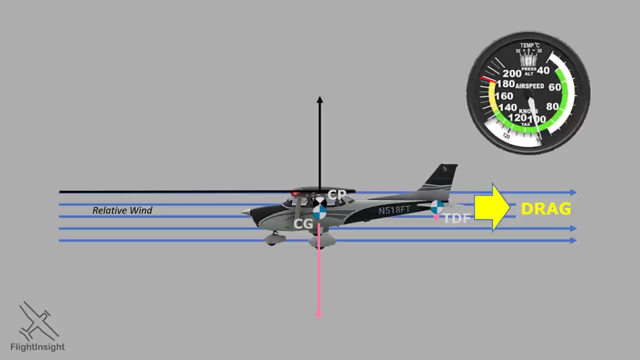 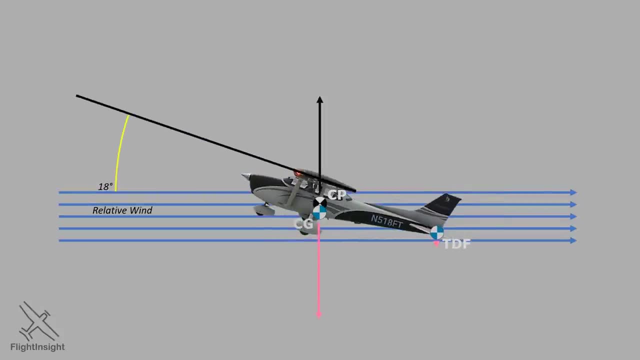 backwards. So what's the catch here? Well, we've sacrificed stability for aerodynamic efficiency. It'll be easy to pitch up to our stall line. but it's not going to be easy to pitch up to our stall line. We're going to need to adjust the angle of attack now that we're not as nose heavy When the aircraft does stall, though that lack of weight up front will mean the aircraft won't pitch down as easily in the stall. Recovering from the stall will be difficult and may take more elevator authority than we have to accomplish, making the aircraft much less stable. 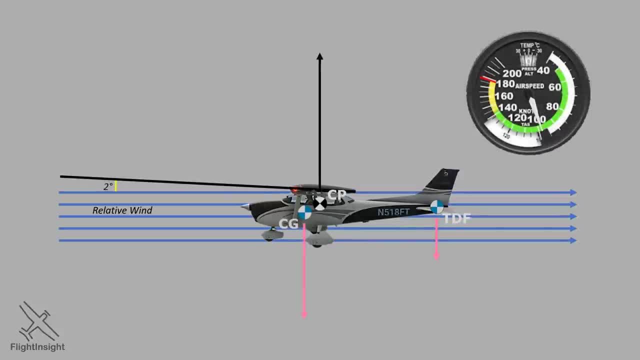 What about stall speeds? We know the color coding on the airspeed indicator shows us that the bottom of the green arc is our stall speed in a specified configuration, which we can see in the aircraft POA. in this configuration, In fact, the green arc on the aircraft POA indicates that we're 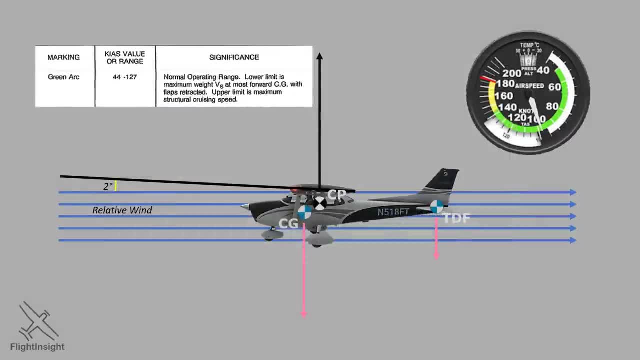 at the bottom of the green arc. If we look at the green arc section, it tells us that the stall speed will be at the bottom of this arc when we have our most forward CG allowable. So does the placement of our CG affect stall speed? Yes, it does. Let's see what that looks like with the CG as far forward. 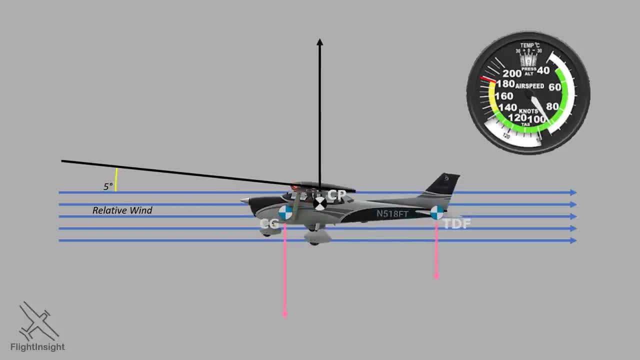 as we're allowed to go. Once again, we'll need a larger tail down force and hence a greater angle of attack. We've already moved closer to our stall angle, which might give you a hint right there If we pitch up to 18 degrees. 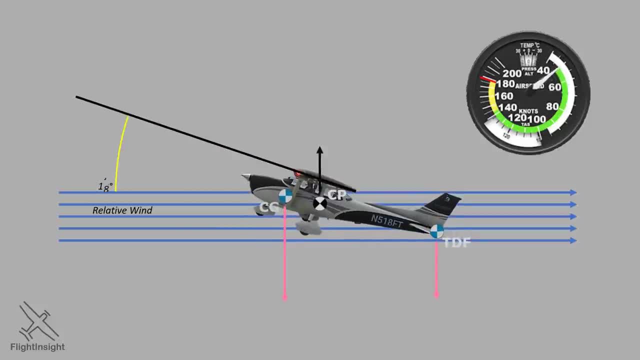 we'll get the stall just as our speed decreases to the bottom of the green arc. Now let's move the CG all the way back to the rear limit. Our angle of attack decreases. We're further away from that stall angle. This means that we have more room to go to pitch up and 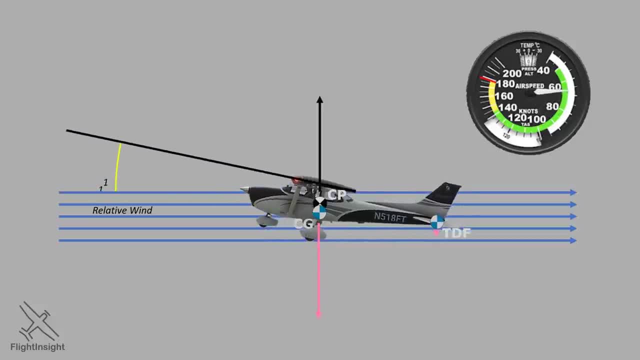 diminish speed before the aircraft will stall, Our stall speed decreases and we'll find it somewhere below the green arc. So that forward CG makes us more stable and protects us in a stall and it also makes us less efficient and or slower And brings our stall speed up. Where we load the weight into the plane, then matters. 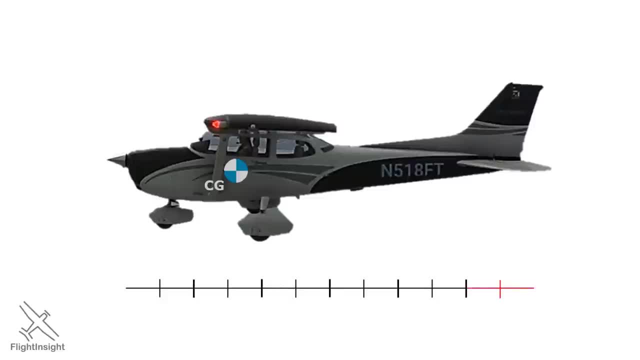 We can define positions on the long axis of the plane, called arms, based on their distance in inches from a predetermined point In the Cessna. that predetermined point happens to be near the engine firewall, So we say that's at zero inches and as the reference datum Any other position on. 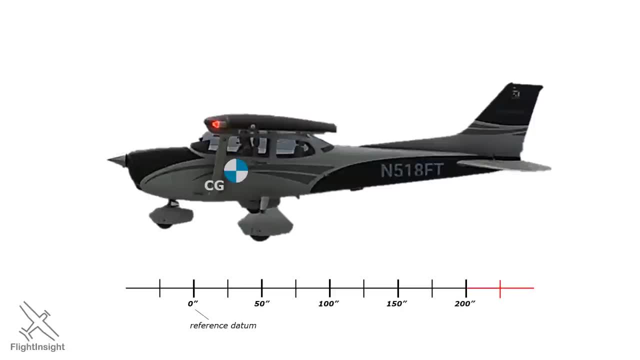 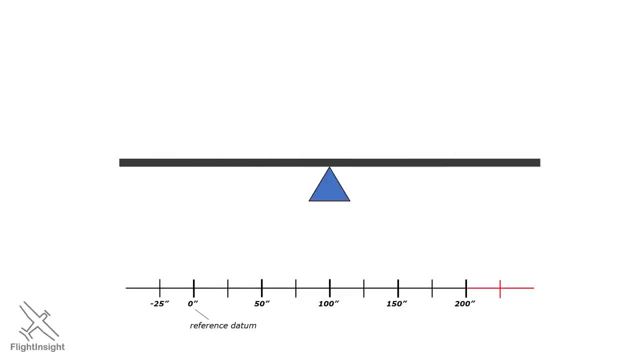 the aircraft is measured as its distance from this point. Anything in front of this point will have a negative number. Anything in front of this point will have a negative number. Anything in front of this point will have a negative number. Let's think of the aircraft as a big seesaw with a balance point or fulcrum in the middle. 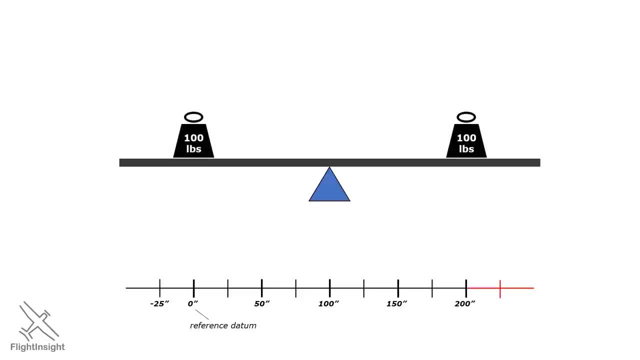 If we load two 100 lb weights onto the plank, one at the zero inch point and the other at the 200 inch point, they'll both be exactly 100 inches from the fulcrum, which is at the 100 inch point. 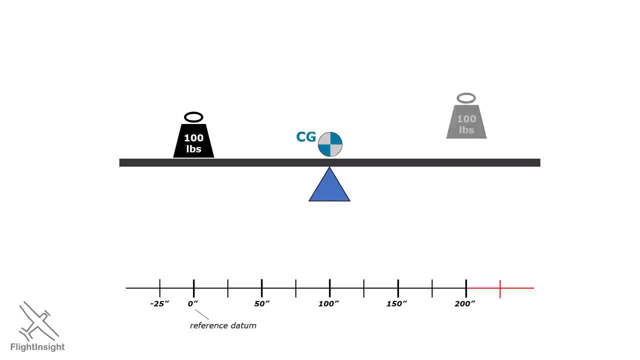 This point is our center of gravity. If we swap one of these weights for a heavier one at the same position in order to balance this plank, now that fulcrum or center of gravity will need to move closer to the heavier weight If we want to bring the CG back to the 100. 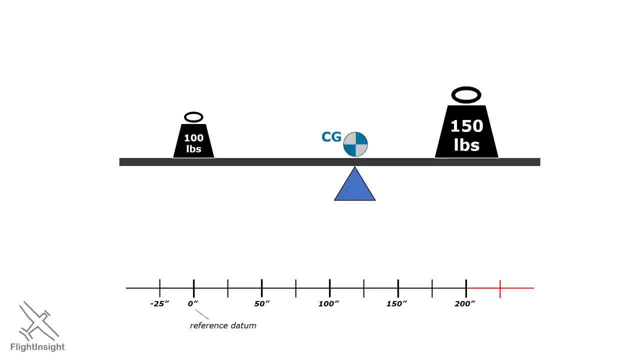 inch point. we could just swap the other weight for a 150 pound one, or we could slide this weight way out till it's hanging over the edge. This will also have the effect of moving the CG point back to its original position. So the lighter weight placed further out. 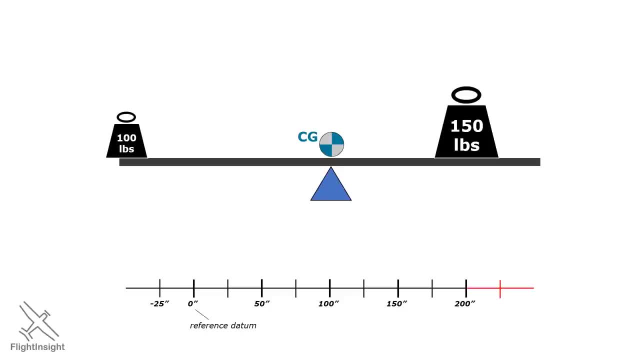 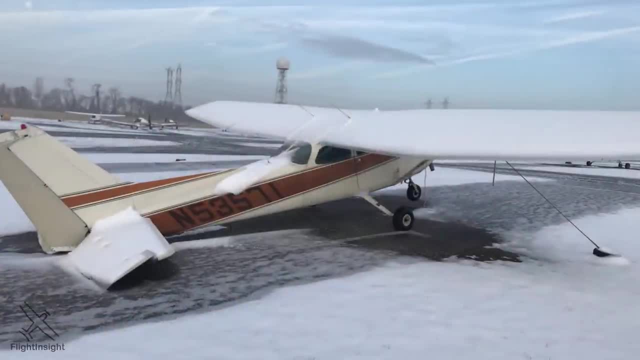 from center will have just as much ability to turn the plank as the heavier weight placed closer in. If this is confusing, consider this aircraft found on the ramp sitting on its tail after a snowfall- The relatively light snow sitting on top of the horizontal. 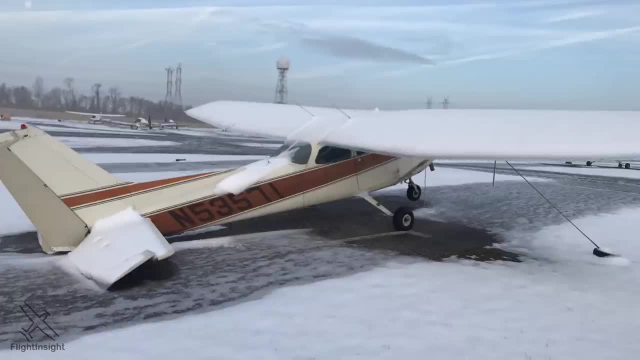 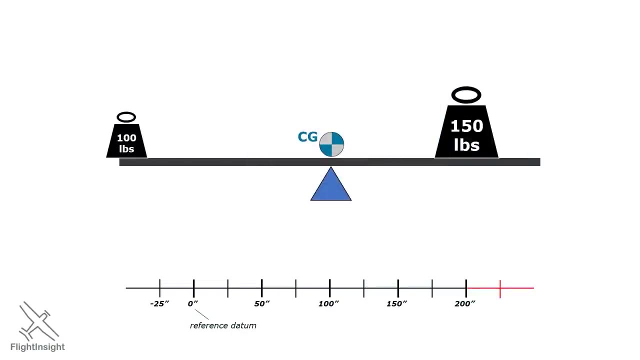 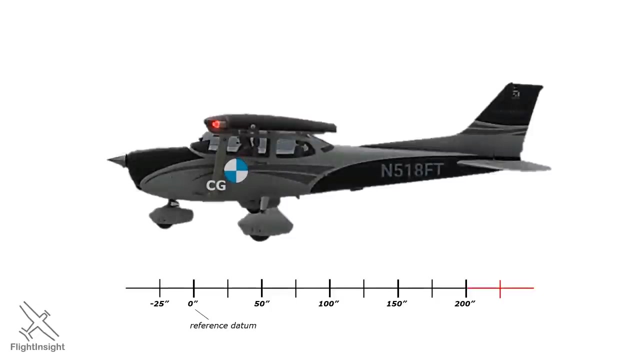 stabilizer far from the aircraft center has a much greater ability to tip it back than that same weight would closer in. One last consideration with center of gravity, Because a well-loaded aircraft has its CG in front of the center of pressure. we usually find the CG to be in front of the two main. 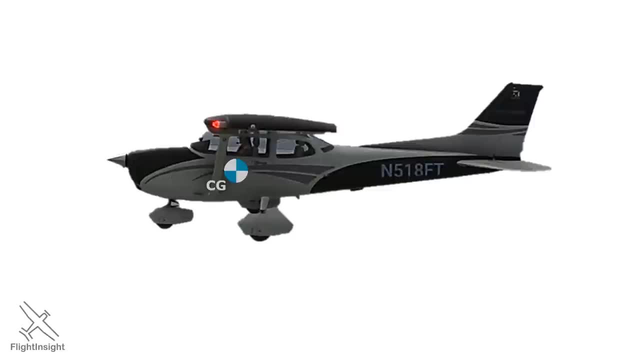 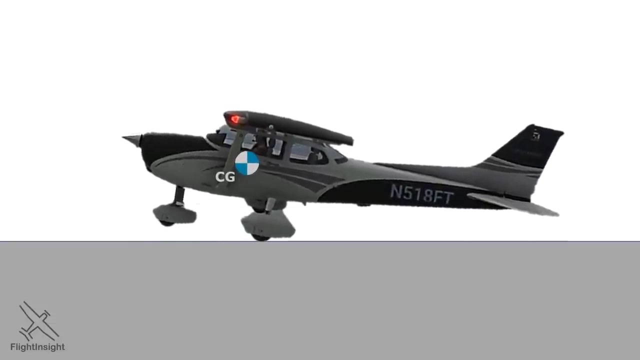 wheels. This doesn't really matter. in flight, The aircraft rotates about its CG in the air, But on the ground, like when we're on the takeoff roll on the runway, the aircraft must rotate about its main gear. This causes it to be nose heavy. We need extra back elevator.